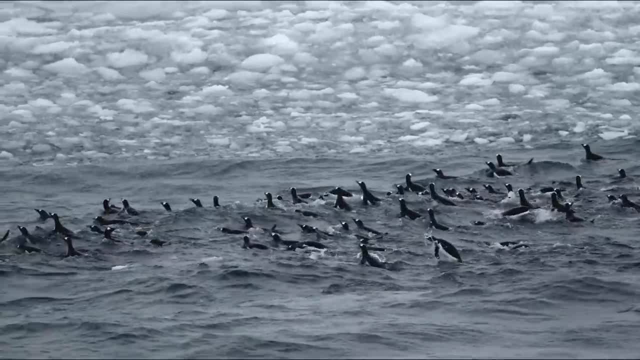 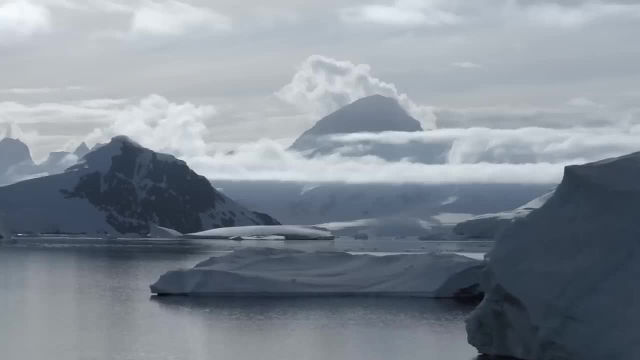 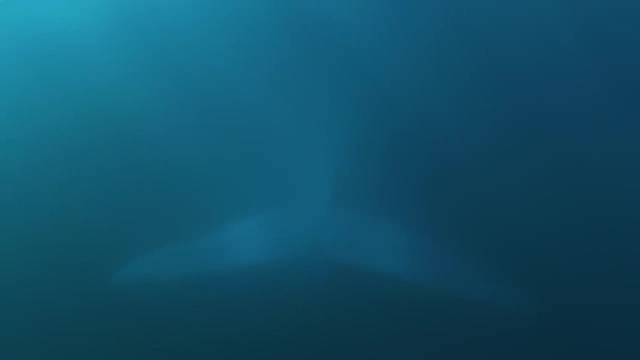 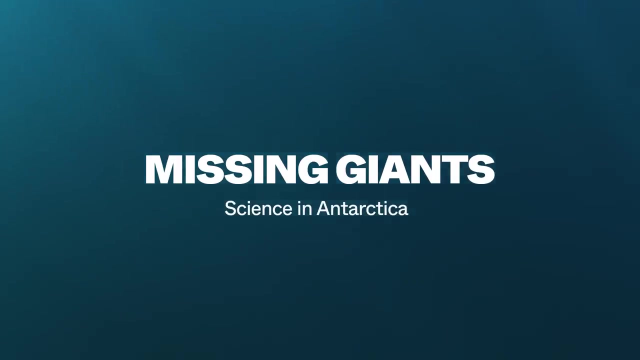 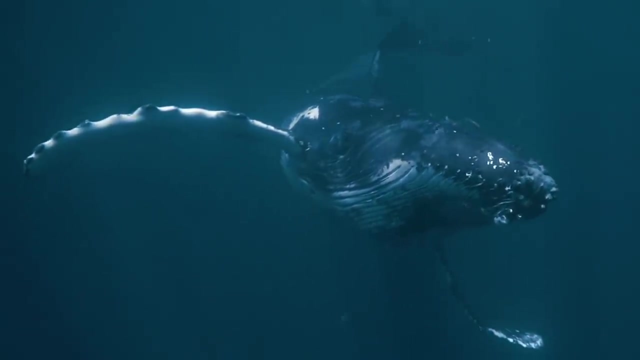 other predators of krill and the krill themselves would explode in numbers. Neither of those things really happened. Krill populations don't seem to have increased since the removal of whales, but actually decreased. My name is Matthew Sivoka. I study large marine animals and, in particular, baleen whales. 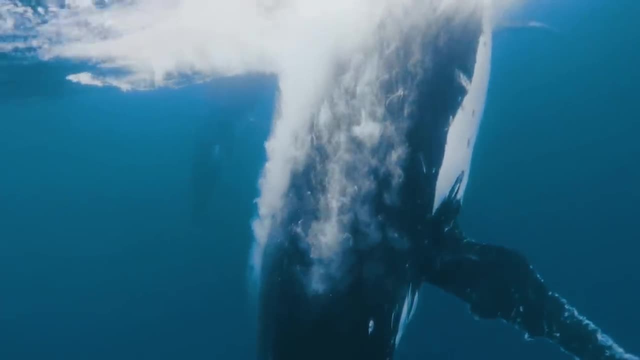 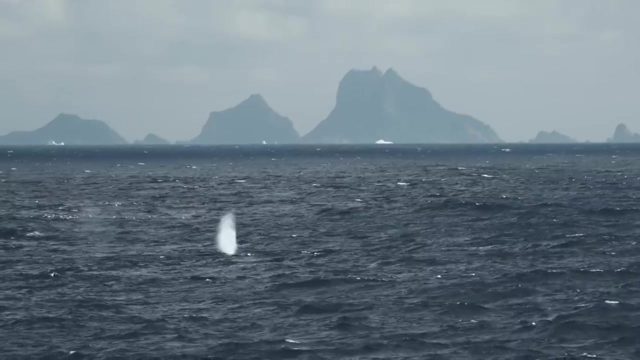 These are animals that are as large as commercial airliners, and yet we don't know their most basic biology. That's what we set out to do by just asking a simple question: How much food do these large whales need? Without knowing how much food they need, then we don't really. 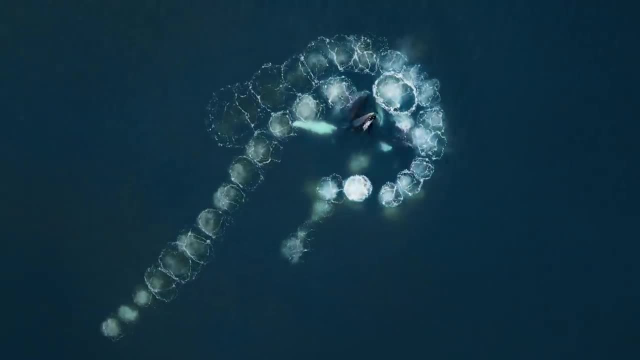 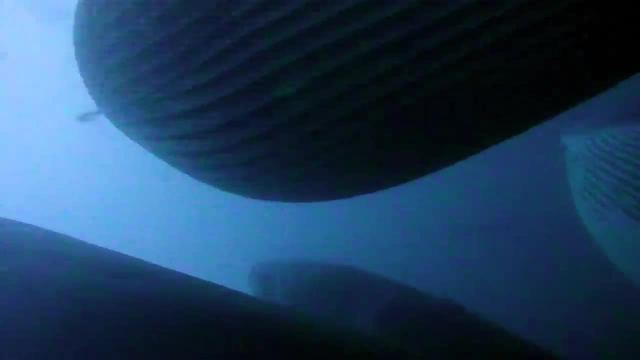 understand how these ecosystems work, how much prey might be out there in the ecosystem to support the number of whales that we know exist in that ecosystem, And for this study in particular, there were three main techniques. The first was to find out how much food these. large whales need. The second was to find out how much food these large whales need. The third was to figure out how to localize, stomach them, landing them in a tupperware or even a shipment. And what else do these huge whales need? And we talked to researchers. 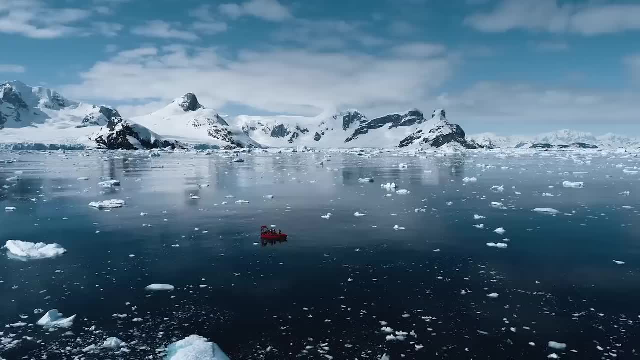 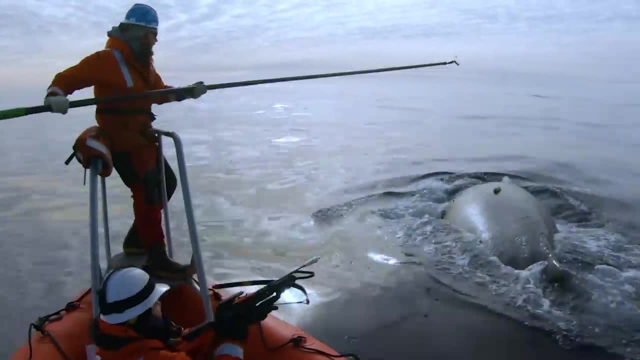 atiento technologies that we took use of. The first is high resolution movement sensing tags- Basically these whale iPhones. They have high-resolution accelerometers, magnetometers, GPS cameras, light sensors. We put it right on the back of a whale and it can then travel with the 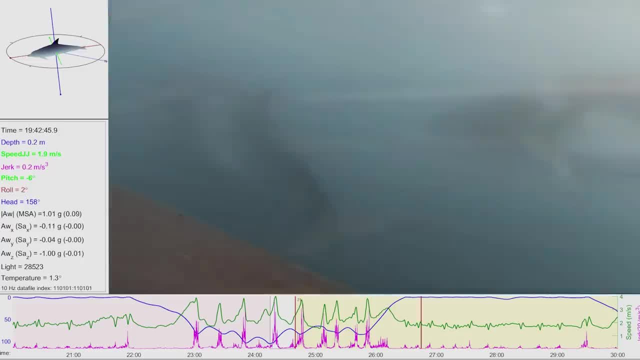 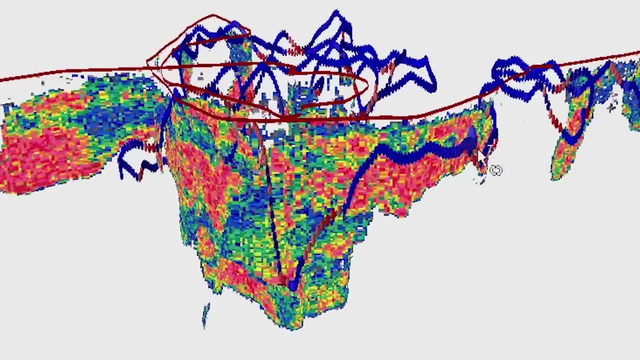 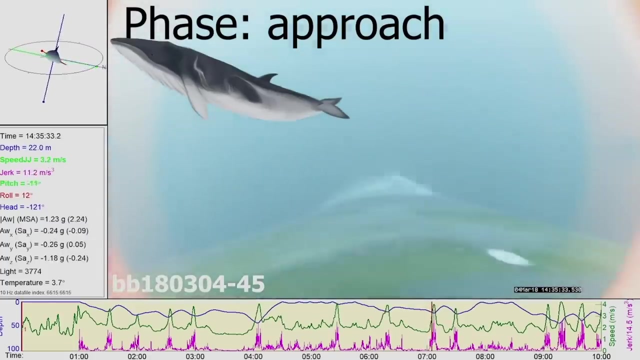 whale several hundred meters underwater and can stay on the whale as long as a couple days. We can take the data from these motion sensors on these tags and then reconstruct not just their movement path but their behavior, production behaviors. And that has been a real breakthrough in understanding whale ecology because before 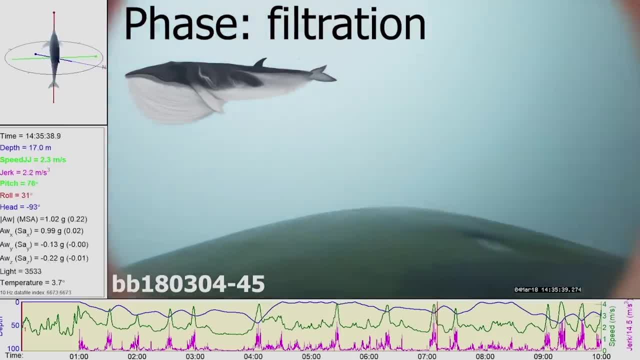 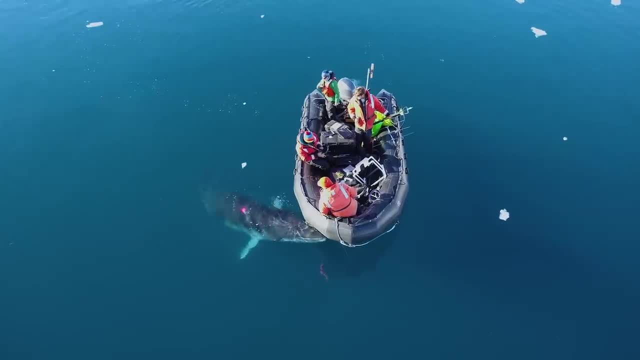 the advent of these tags, we didn't really know what they were doing underwater. The second bit of technology are drones. When we tag a whale, we like to measure that whale. Once we measure the size of that animal, we can relate that to the size of the mouth, how big of a gulp of water? 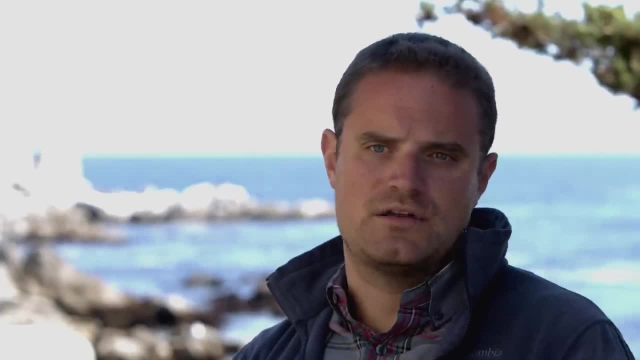 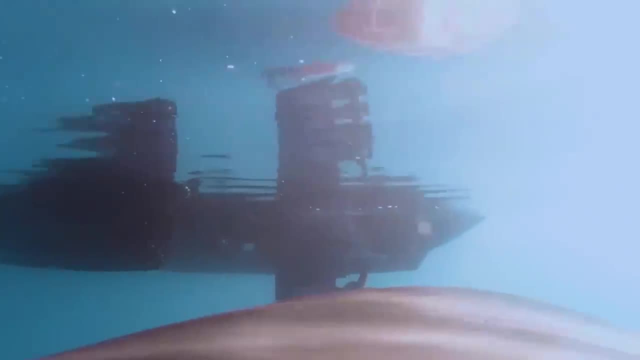 they can take. You have the tag which tells you how many gulps of water they were taking in a given period of time and the drones which can tell you the size of each of those gulps. The last component is using echo sounders to figure out the density of those krill swarms. 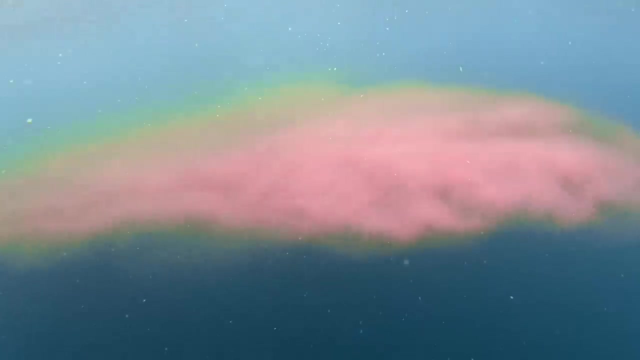 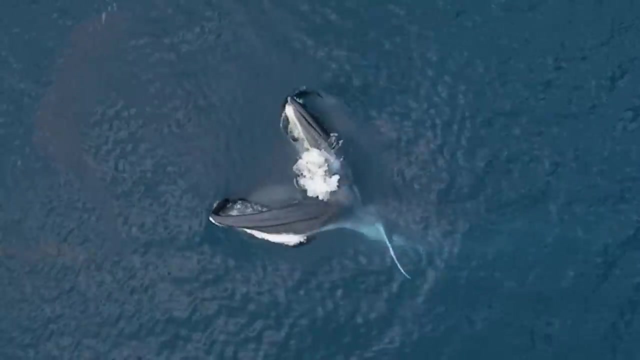 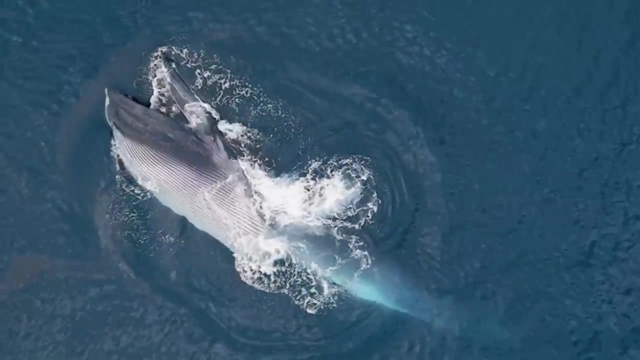 Putting those three things together, we can figure out how much these whales are eating per mouthful, per dive and per day. Large baleen whales only eat about 50 to 100 days a year, And then for the rest of the time they just don't eat, unless there's enough. 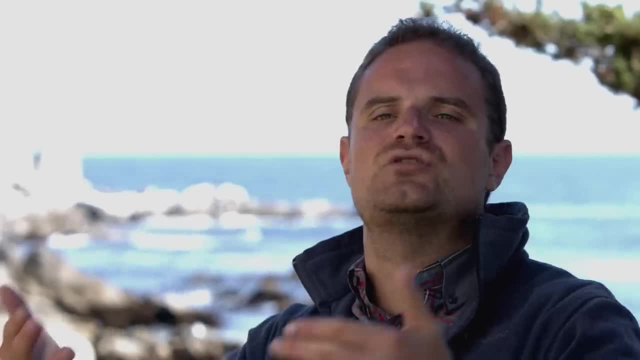 corn to feed them, And then for the rest of the time they just don't eat unless there's enough corn to feed them. And then for the rest of the time they just don't eat unless there's enough krill per cubic meter of water. then these whales will actually lose energy eating. 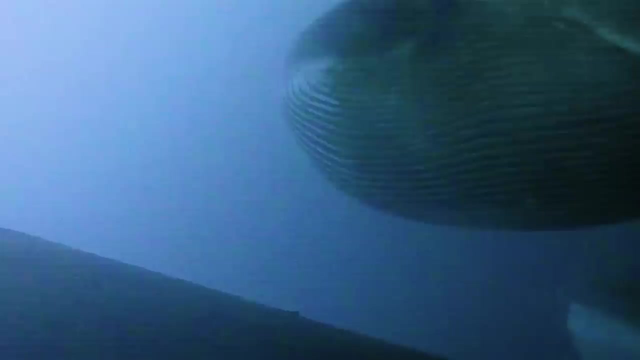 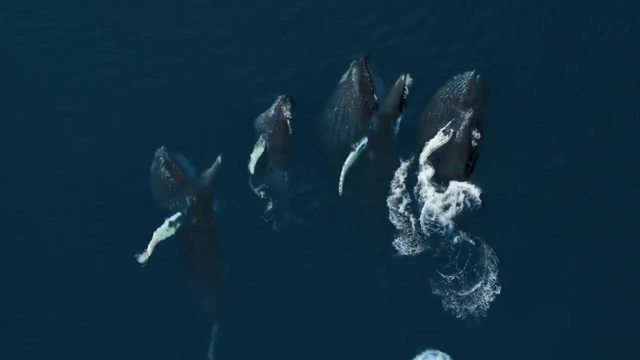 The amazing thing is they do this hundreds of times a day. Imagine eating a buffet while running three marathons back to back to back. That's what a day in the life of a feeding whale is like. Before the use of this technology, I don't think anyone really expected them to be. feeding that much. Just the quantity of what they eat is astonishing, Sometimes three times higher than we expected, As much as four times higher than we expected, And then for the rest of a day, We're able to feed about four, five, six tons of krill a day. 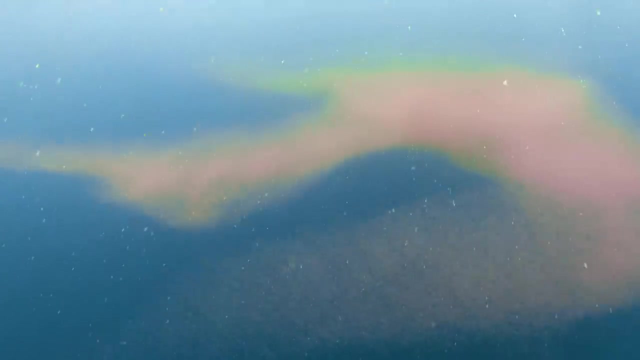 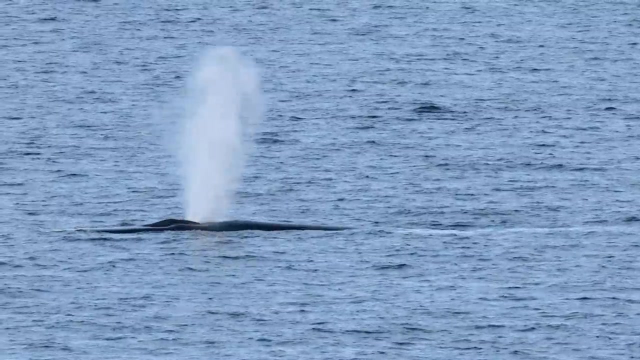 Therefore, the quantity of what needs to be in ocean ecosystems to support them is also large and important. It makes us re-think and reframe how ocean ecosystems work, how we should manage them, not just for whales, but for people as well. 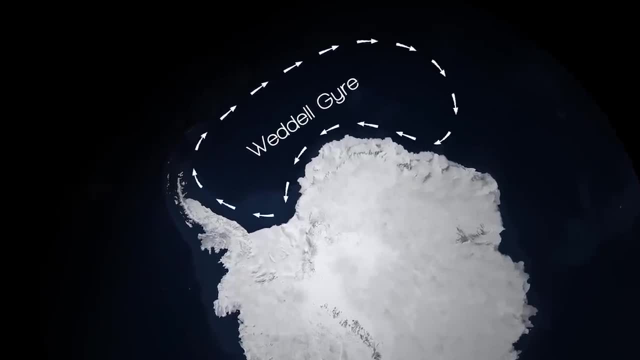 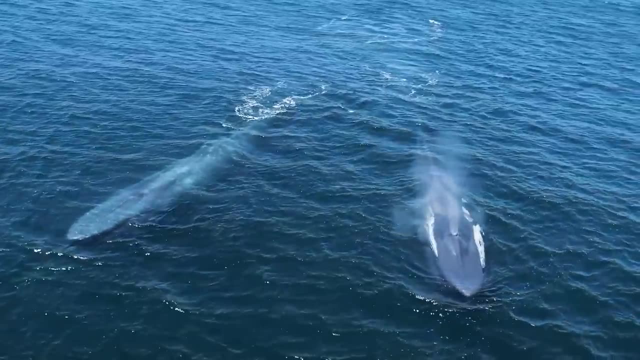 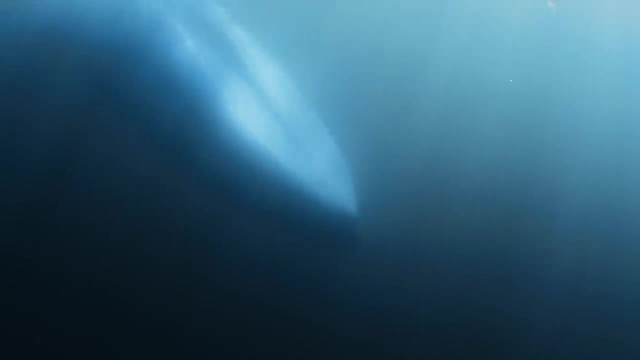 The Wannel Gyre is the largest oceanographic feature in the southern ocean, where by far the most whales were and by far the most krill was and is, and we estimate that just the blue and the fin whales there ate roughly 100 million tons of krill there each year prior to whaling. we don't know. 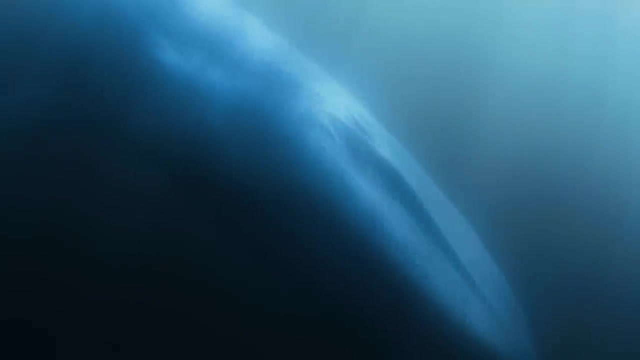 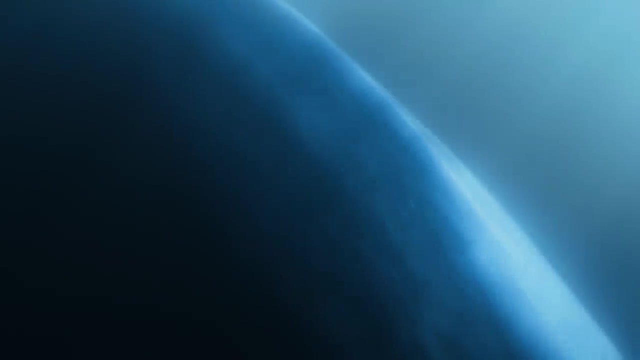 exactly how much krill was in the system then? possibly as much as 500 million metric tons just in the weddell dryer system alone. now in the weddell dryer system there's about 60 to 70 million metric tons. the difference between these numbers is so stark that even if our estimate for 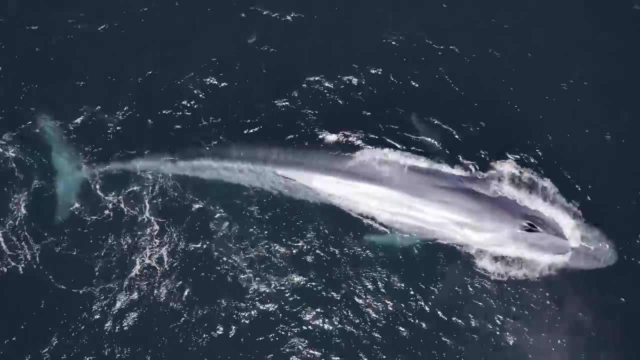 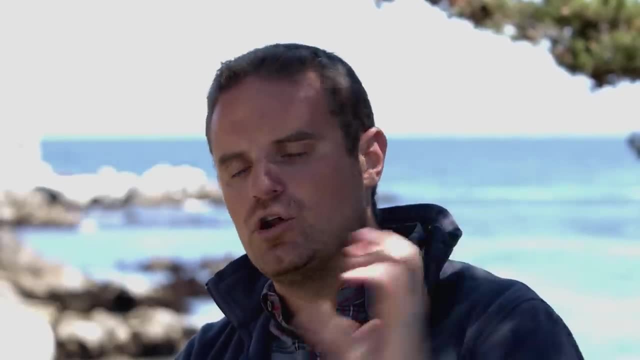 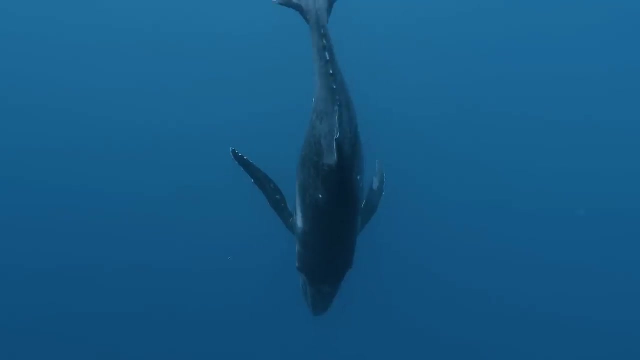 how much whales eat are off by two or threefold. there's still not enough krill in the weddell dryer to recover whale populations to even close to the level we're at pre-whaling. how can we understand the collapse of krill stocks? first, we need to look at ecosystem dynamics. whales- 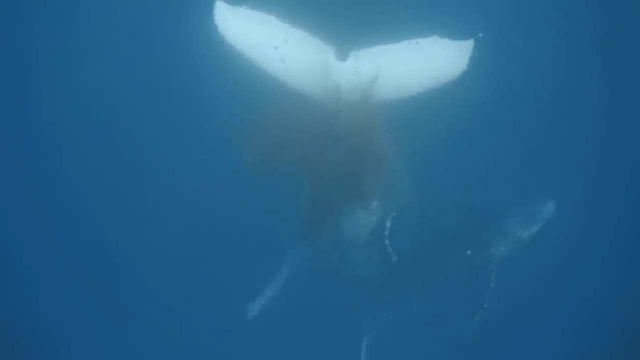 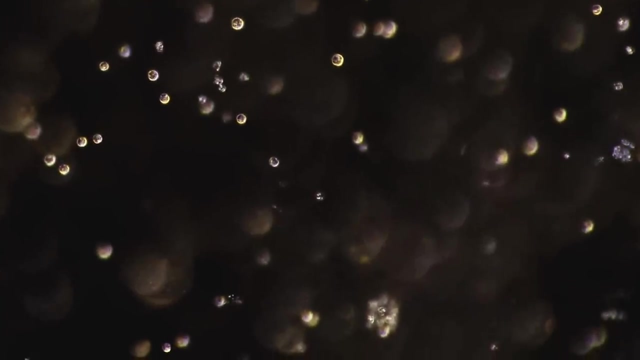 act as mobile krill processing plants. in the summer, in the southern ocean, in particular the whale food web, you have whales that are feeding on krill and krill that are feeding on phytoplankton. the phytoplankton need nutrients to grow. they need iron. 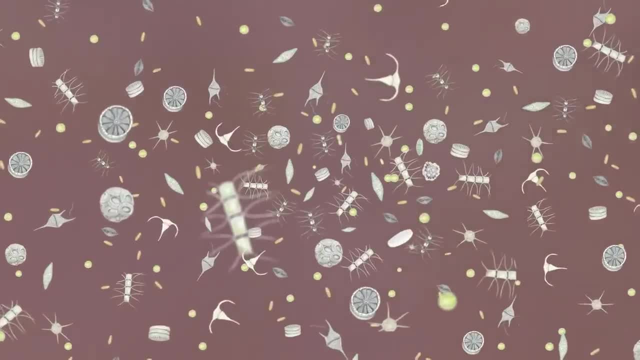 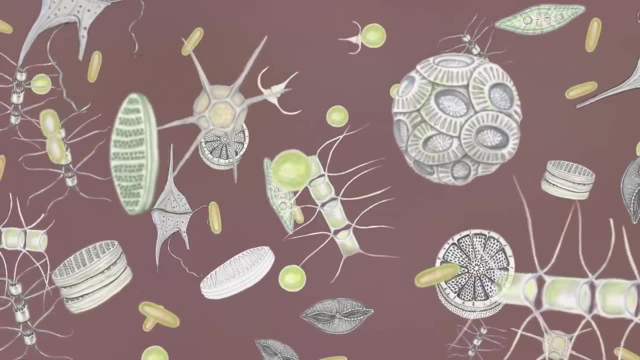 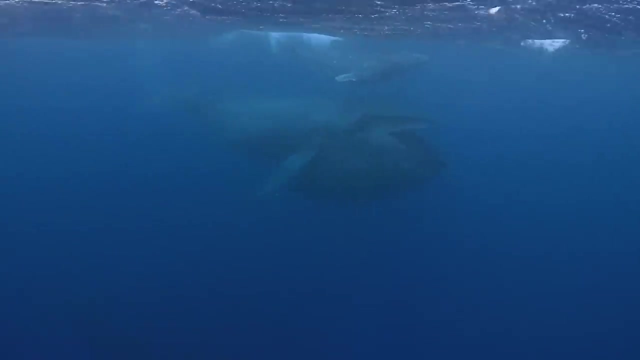 iron is abundant in whale poop. whales eat krill and they poop out iron-rich feces. the phytoplankton draw in that iron to build those communities of phytoplankton which then feed the krill, which then feed the whales. essentially, whales create pastures in the sea that the krill 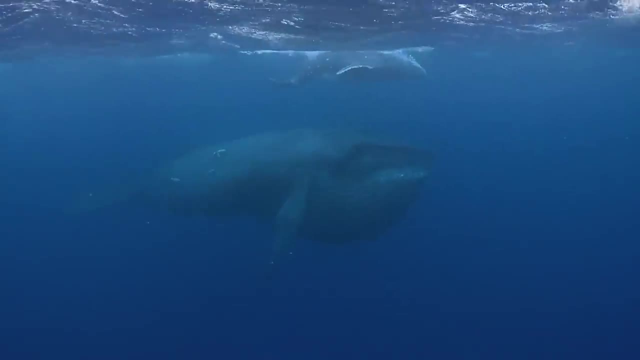 use to eat to thrive. the whales and their prey, the krill, were actually locked in this mutualism where they both need each other. the whales need the krill just as much as the krill need the whales. when we removed the whales, we pulled the plug on this ecological mutualism that really held this. 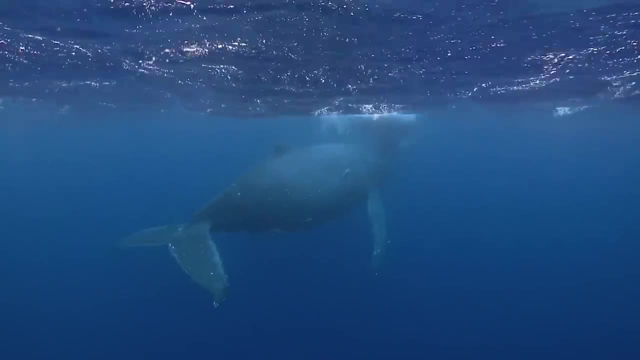 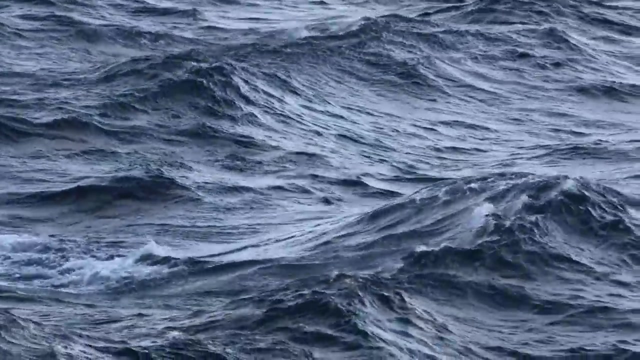 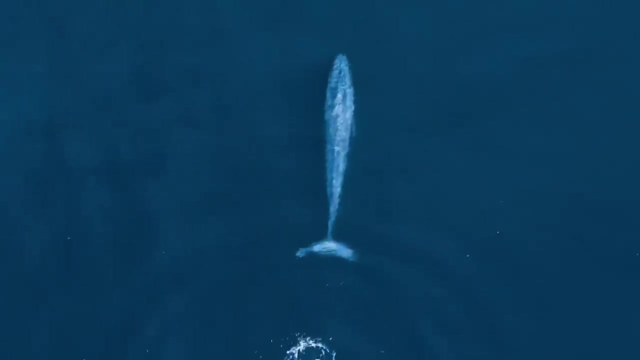 whole ecosystem together, and that system has since fallen apart. right now, most of the weddell dryer is a biological desert. we believe that the removal of whales drove this initial decline, and climate change is limiting its recovery. on top of that, we're competing with the whales for the krill that remains. 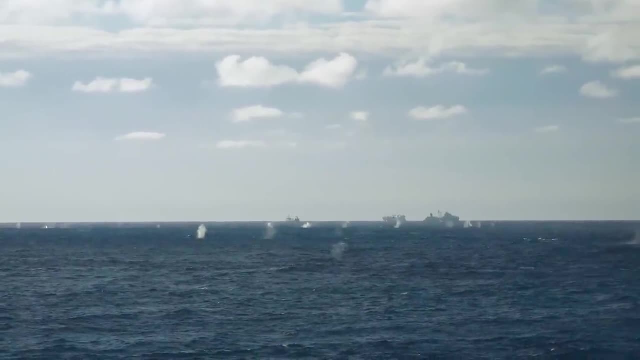 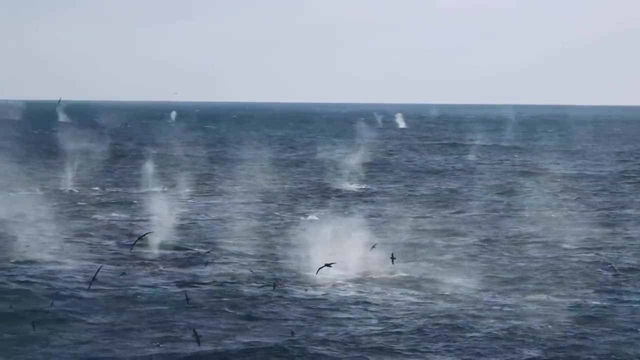 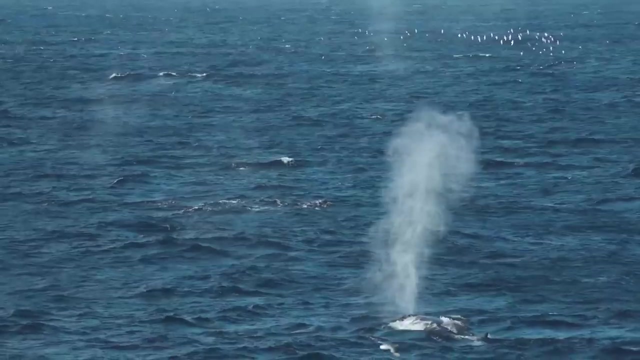 krill fishing is happening in the southern ocean even today. now we are harvesting only one percent of the krill population in that area where this krill fishing takes place. that seems completely fine, and it is, if your goal is to just have that population be replaced year after year. but 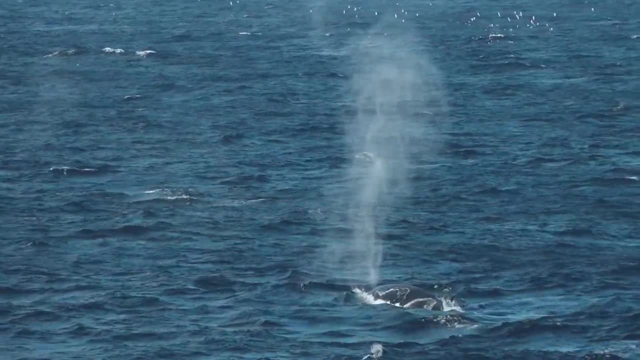 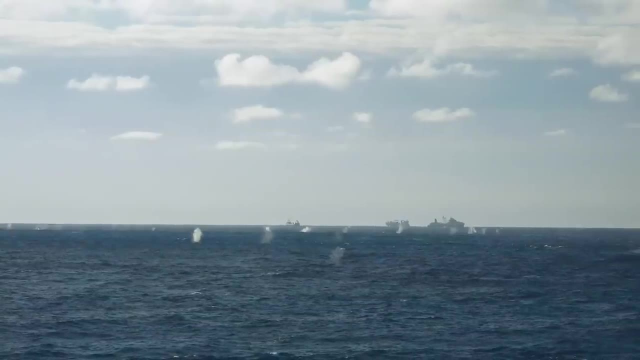 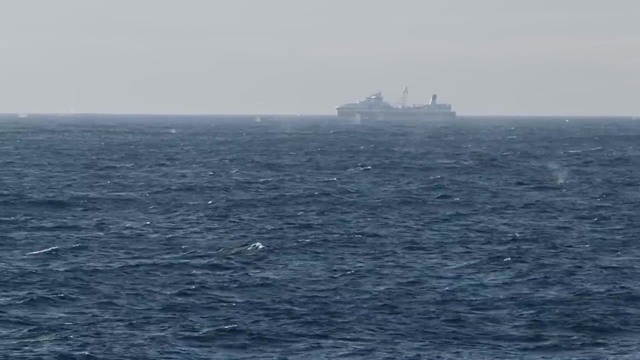 if you think about the importance of krill to antarctic predators, even the removal of half of one million tons of krill, if it overlaps in space and time with these krill predators, could be very detrimental. if krill swarms get large enough and dense enough, they become immensely valuable to 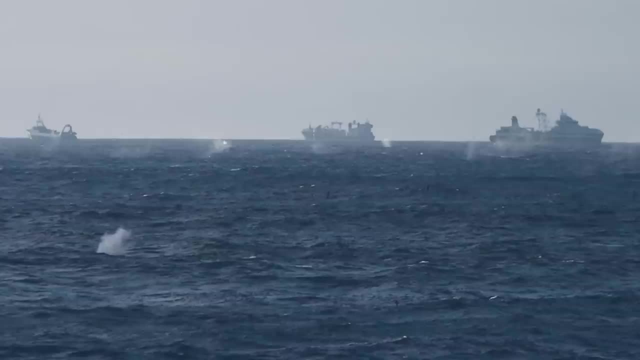 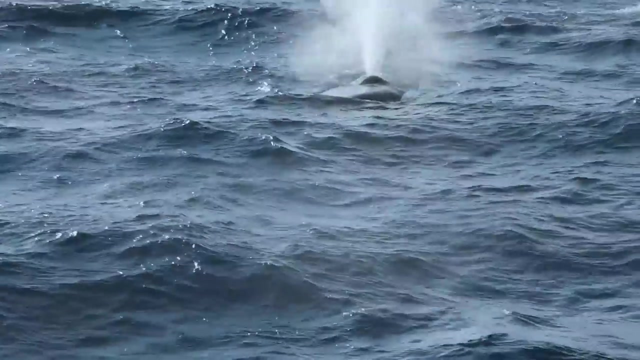 whales and they're also quite uncommon. the issue is as management currently stands. those are also the patches that are the most valuable to the krill fishery, these hyper-dense clays of whales, patches of krill, the same very patches that we know these whales are feeding on and are dependent. 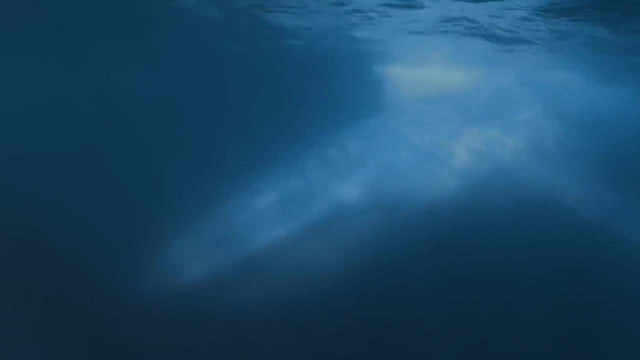 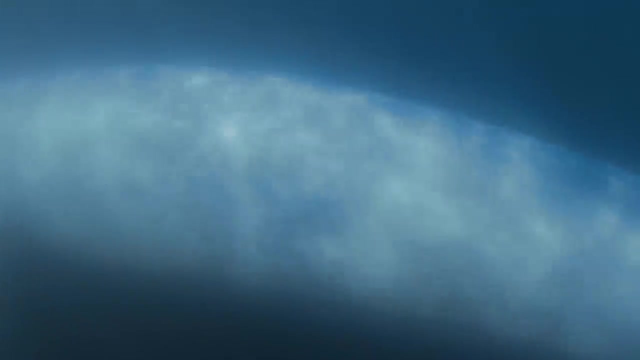 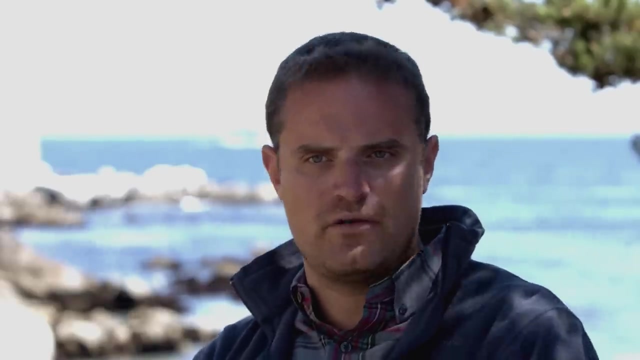 on to survive and reproduce. it's easy to break an ecosystem and it's very hard to put it back together. if we want to rebuild whales to anything even remotely close to what we saw before whaling, we need more krill period. that's. it's just simple math. it became quite clear we really need to stop. 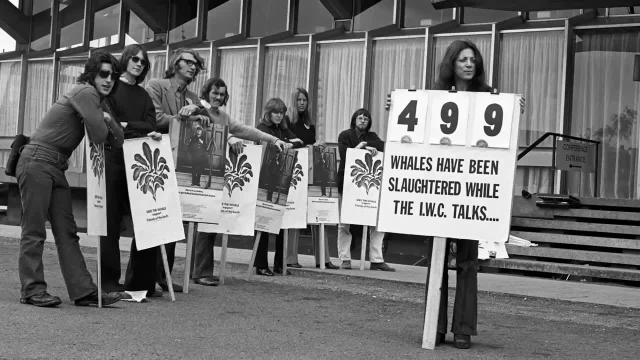 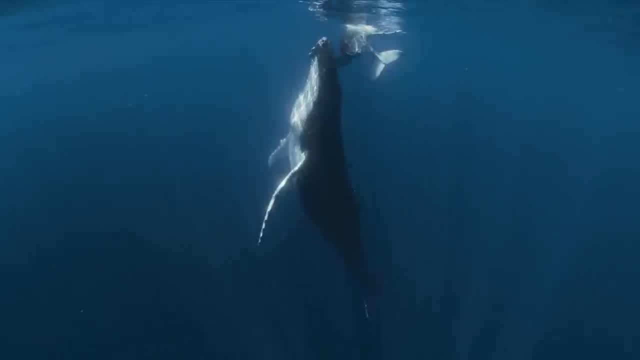 hunting whales altogether at this industrial scale, if we want whales on the planet at all, and so in the early 1980s, there was a global whaling moratorium. since the moratorium, humpback whales around the world are recovering extremely well, so this is something that we need to. 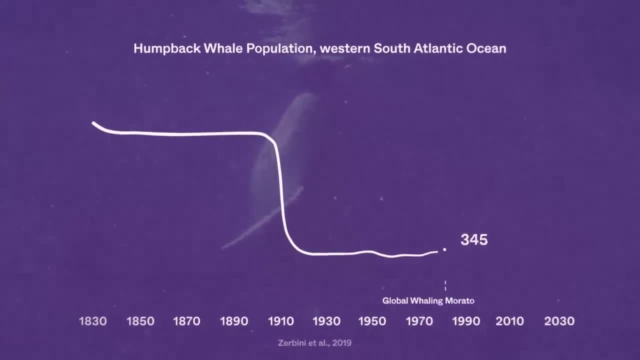 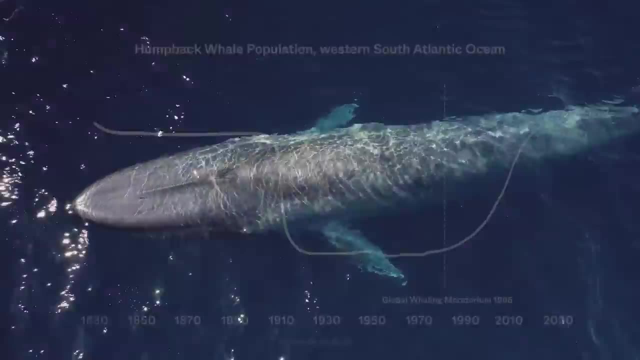 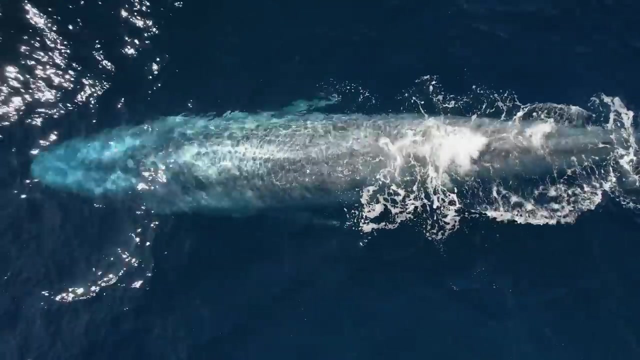 celebrate. these conservation measures do work, and humpback whales are a great example of that, but unfortunately other whales are not doing so well. antarctic blue whales are still at about one percent of their historic population size 60 years after we stopped hunting them. what you can lose in 50 years. 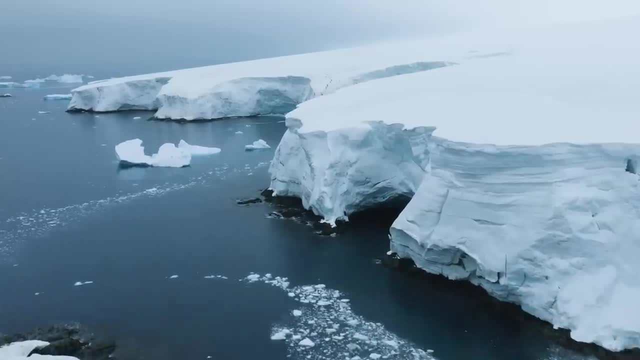 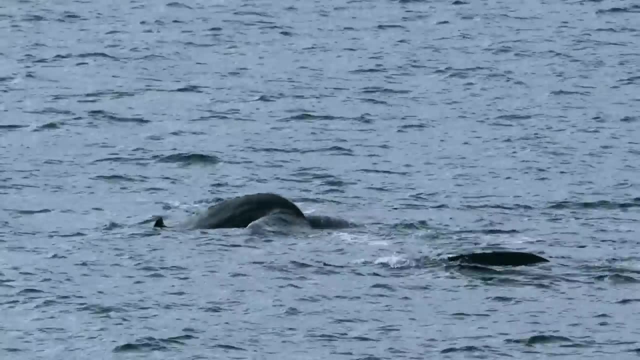 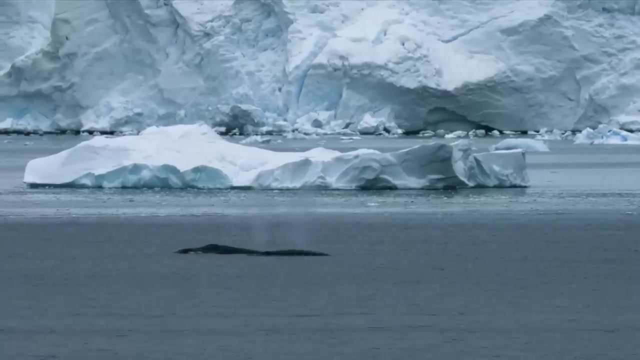 might take 500 years or more to grow back. we need to think really carefully about how we protect these resources moving forward. if we bring back whales, the whales will help us bring back the krill, and that's the situation we all want, whether we're a penguin or a whale or a person. this is 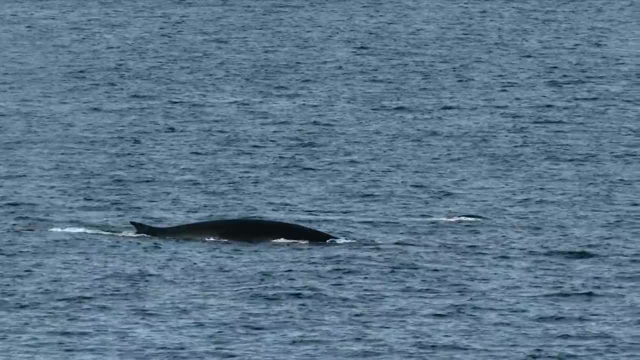 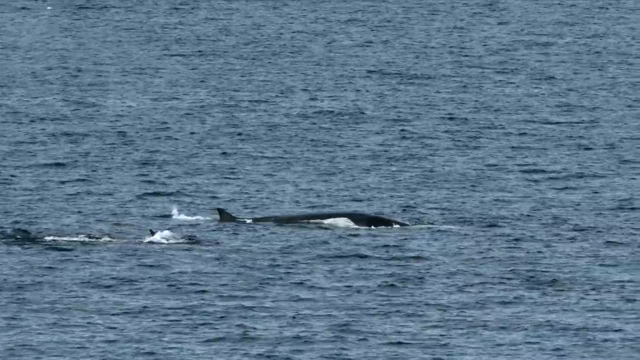 important in the fight against climate change. once carbon is brought into a whale's body it's locked in, in some cases centuries. krill are also super important in the carbon cycle because they have really fast sinking fecal pellets which sink and lock that carbon away to the deep sea. 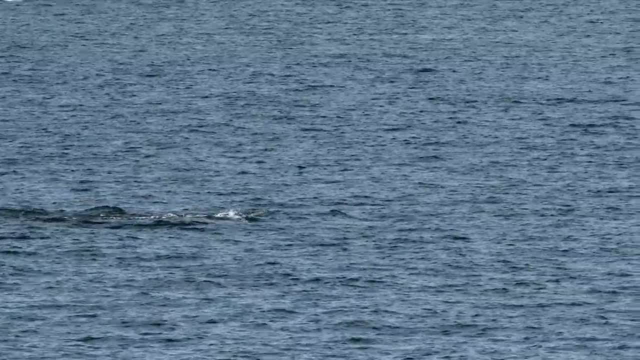 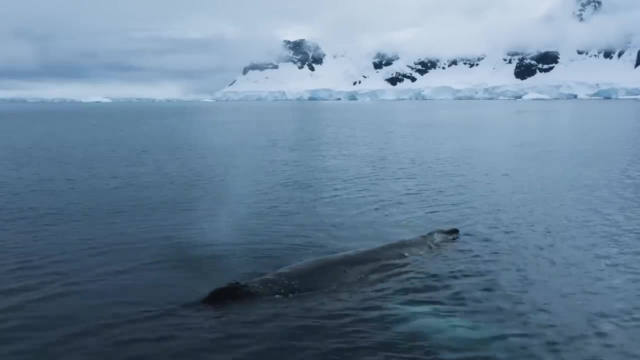 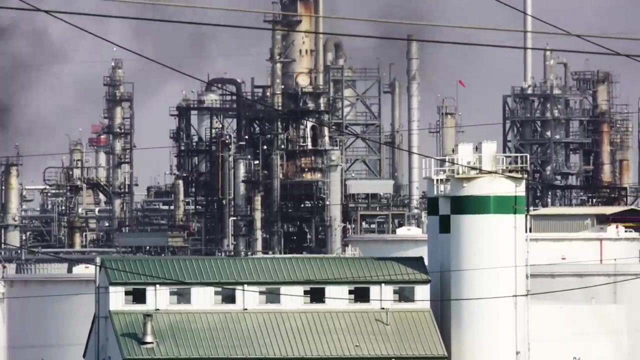 this process of rebuilding whales and krill and the phytoplankton, this very simple food chain of the giants, is going to be incredibly important in the 21st century. in storing and sequestering at least a couple gigatons of carbon, we have about one thousand too many gigatons of carbon. 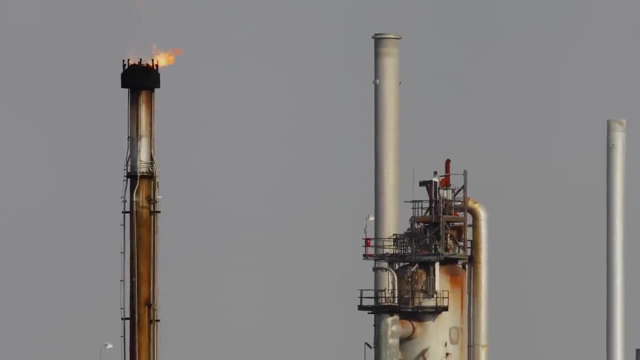 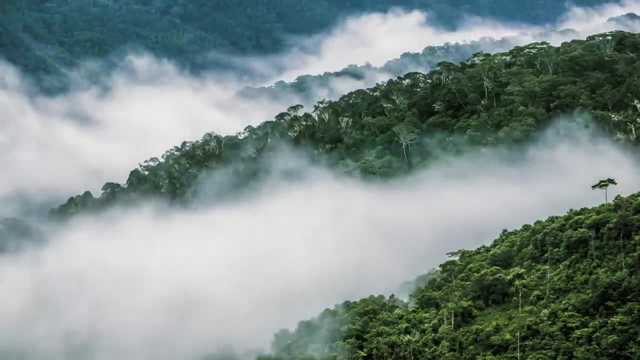 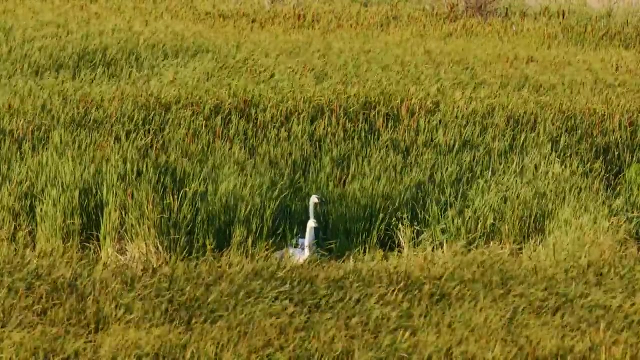 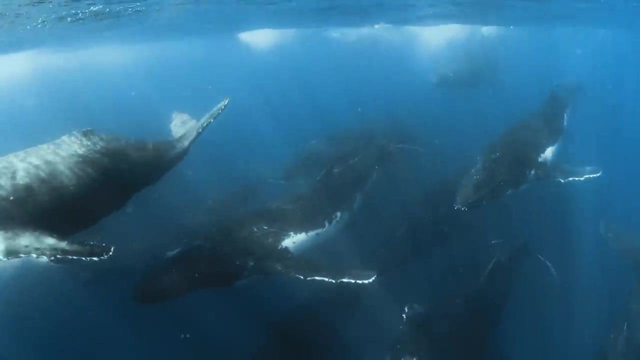 in the atmosphere. so the rebuilding of this ecosystem- will that solve climate change alone? no, but we take all of these natural climate solutions: rebuilding forests, rebuilding fish populations, recovering grasslands. if we consider the recovery of whales and their ecosystems as part of these natural climate solutions, whales are just a slice of the pie, but they are a part. 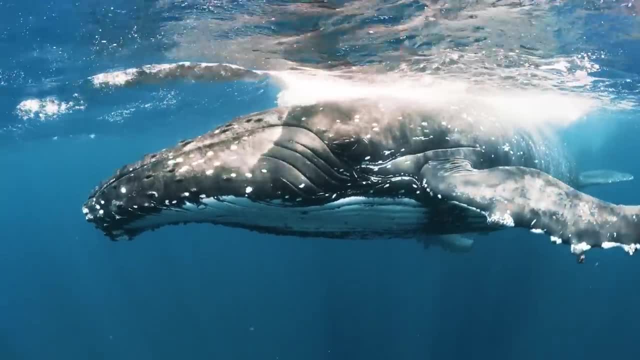 of the pie that we need to consider. if we want to make impacts on large scales, then i think what we need to do is we want to make impacts on large scales, and i think what we need to do is to make is share this message of hope as widely and as quickly as we can.